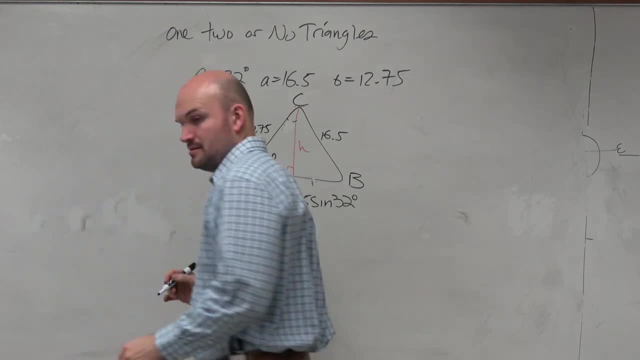 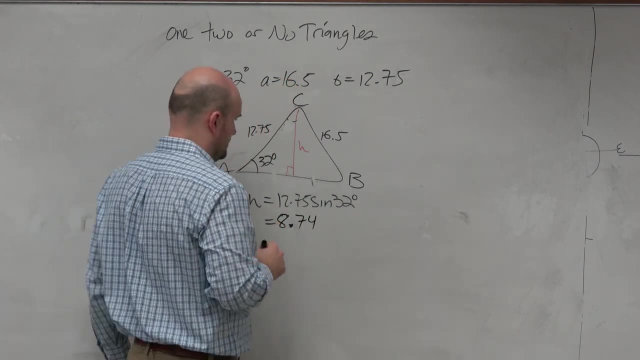 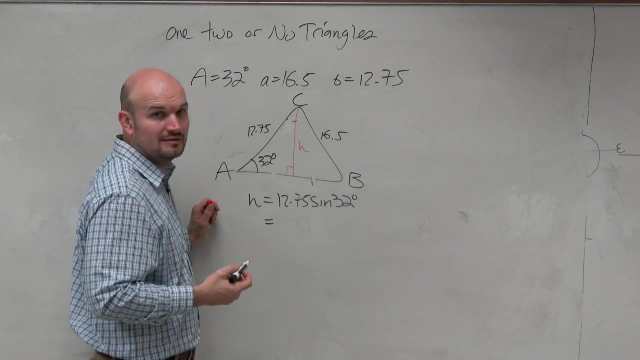 Okay, So H is what H is: 8.74.. 8.74.. I got 6.756.. Uh-oh, Uh-oh, It doesn't matter. I mean it does matter 2.0, if it's one person triangle. 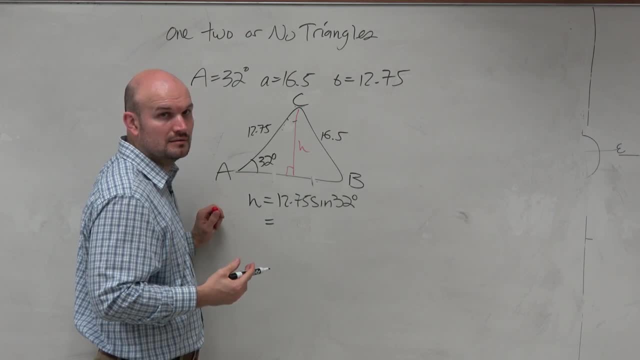 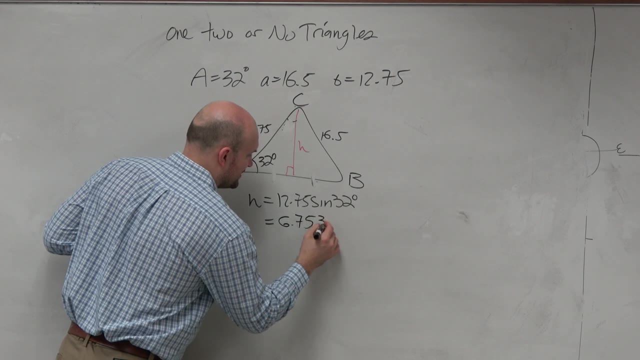 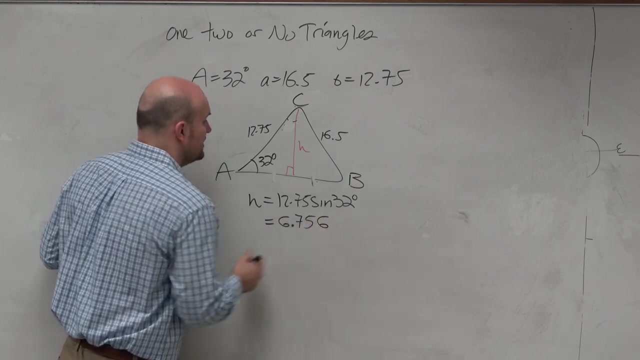 It does, But if it's eight, it's still Okay. well, which I mean? It's 6.753.. 6.753. 6.753.. Oh, okay, Okay. Then again, guys, we can compare this. 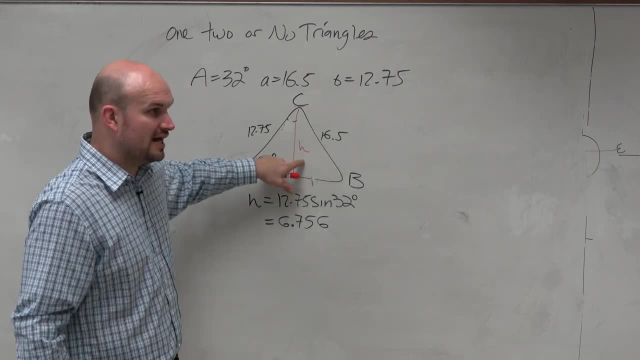 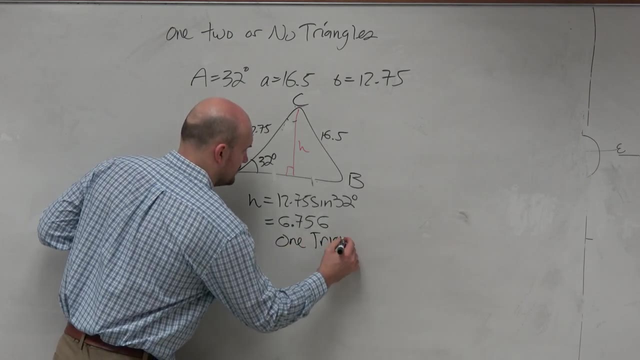 We see that this length is larger than the height, but since it's also larger than my other length, then I know that there's going to be. one triangle exists Right Now. let's say you're taking a test and you're like 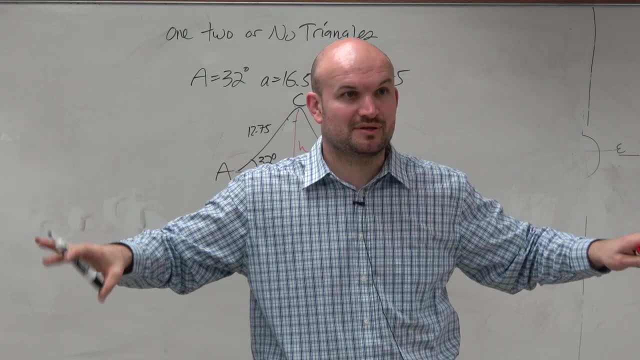 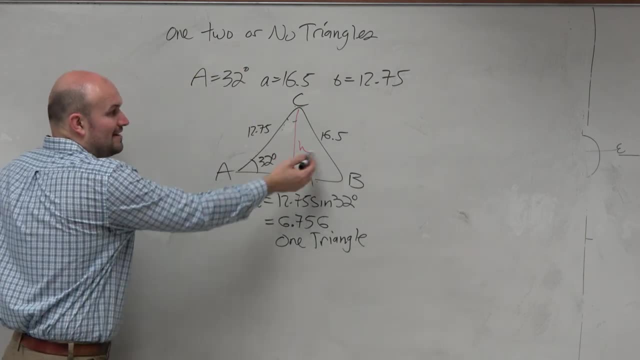 I totally forgot what I need to do because I was playing on my phone when Mr McLeod was teaching this and I completely forgot everything right. So here's another thing you guys can do. We have enough information to do the law of sines, don't we? 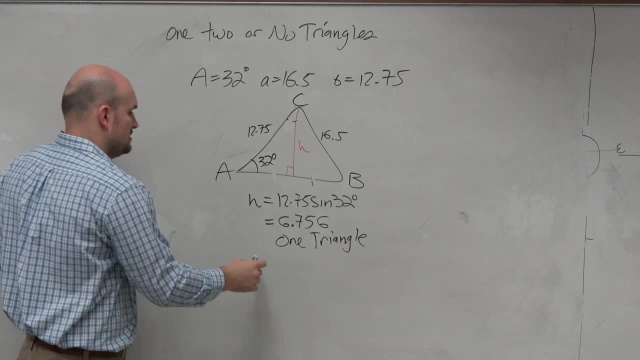 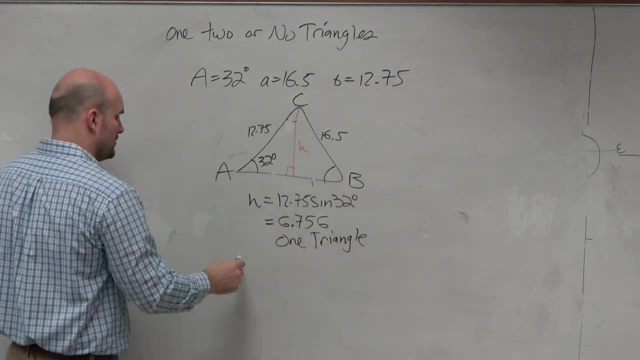 Yes, We have enough information to do the law of sines. So let's set up the law of sines. You know, if we're doing the law of sines, we're going to find an angle. So therefore I can do sine of b over 12.75.. 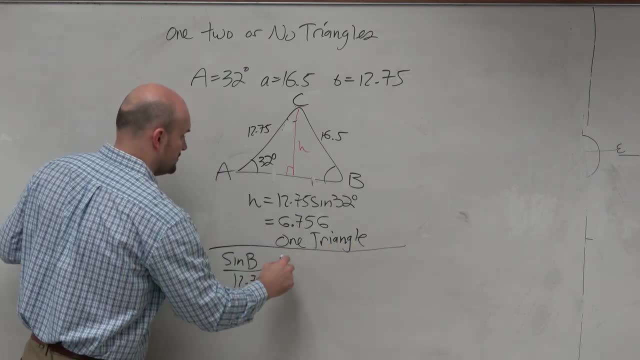 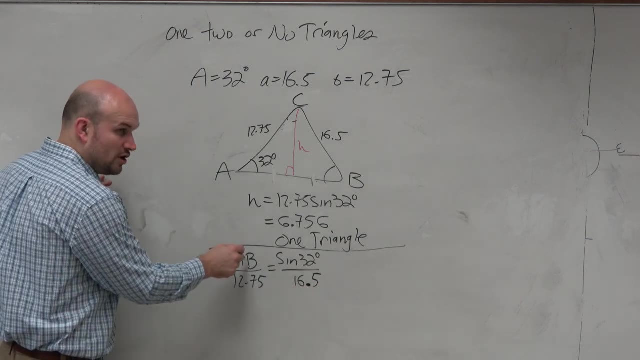 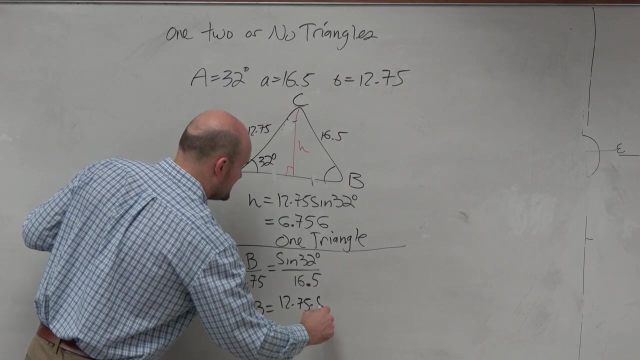 Notice how I inverted them- Is equal to the sine of 32 degrees, all over 16.5.. So now I've got to solve for b, right? So I have. sine of b is equal to 12.75 times the sine of 32. 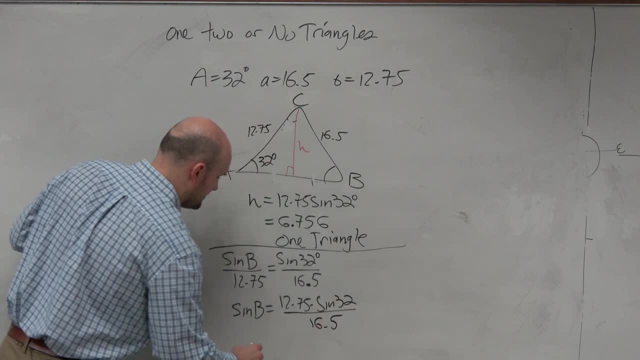 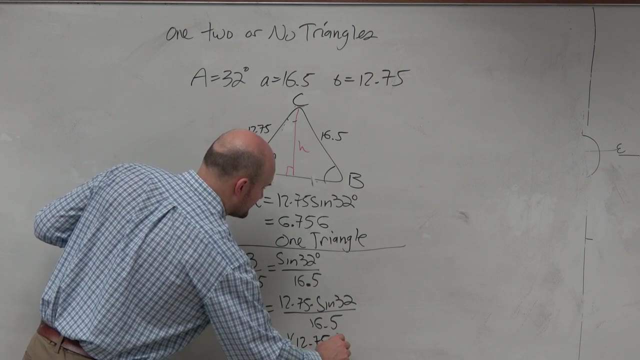 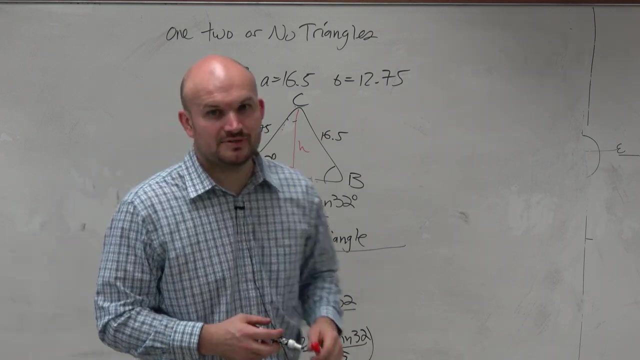 all over 16.5,. and then b equals the sine inverse of all of this. Now, you do not need to write all of this out, I am just writing this so you guys know what to type into your calculator. But that is what you type into your calculator. 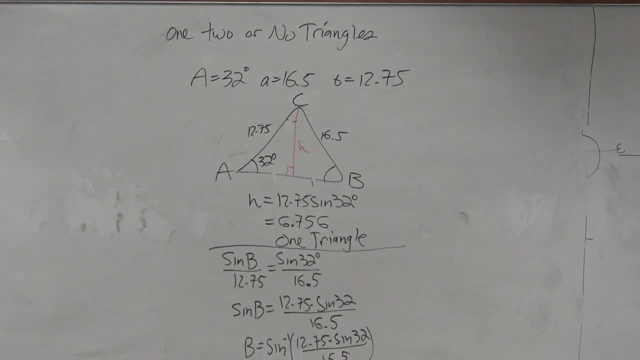 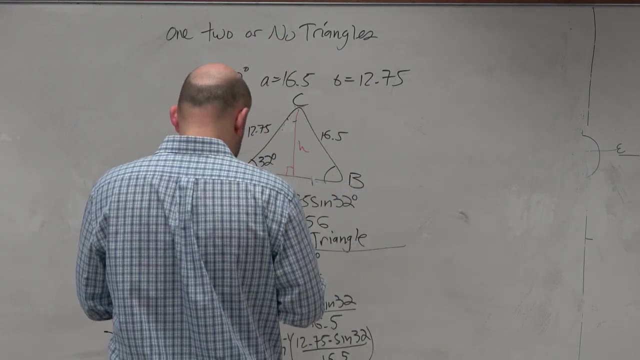 Okay. Now when you type that into your calculator, you get: I'm going to calculate this because I'm so hard to like here, So I'll do 12.75 times the sine of 32.. Close your parentheses. Be careful with that, right. 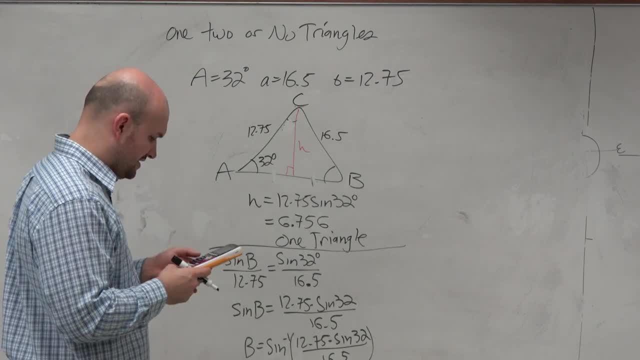 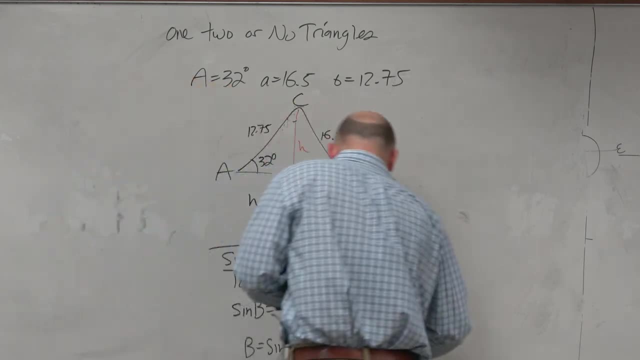 Divided by 16.5.. I'm getting Oops, And then you got to take the sine inverse right. Second answer: I'm getting 24.172.. Anybody second that? Yeah, Okay, Now that's degrees. 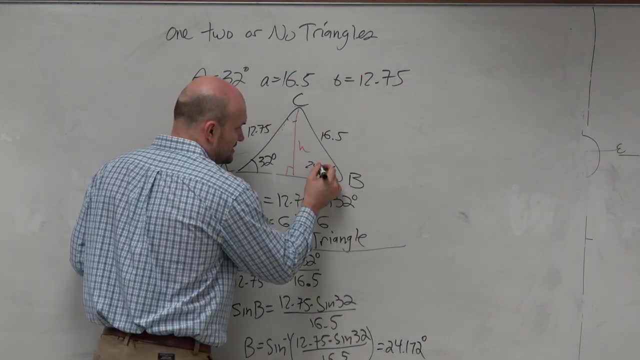 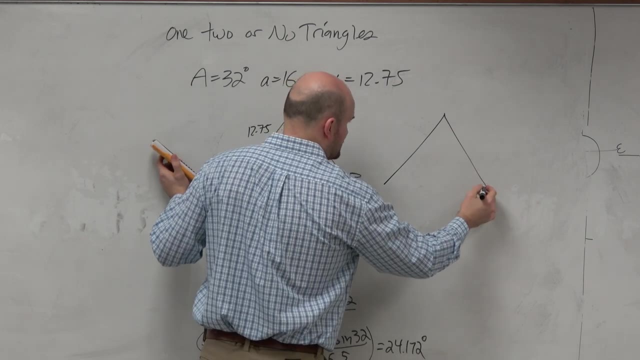 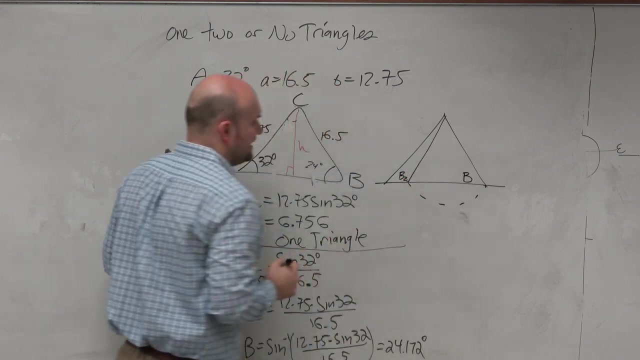 So that means this angle is 24 degrees Right Now. if there was a secondary triangle, right? If there was another triangle, then here's b. b2 would have to be obtuse, right? If this does exist. 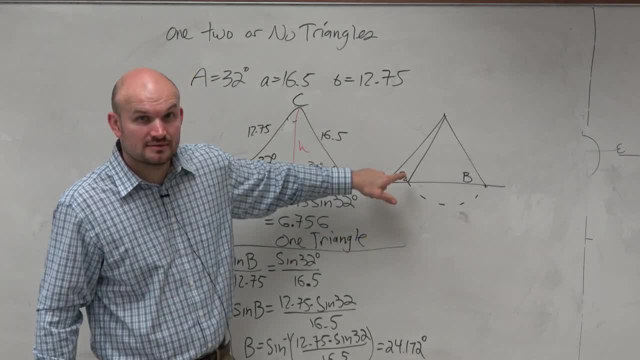 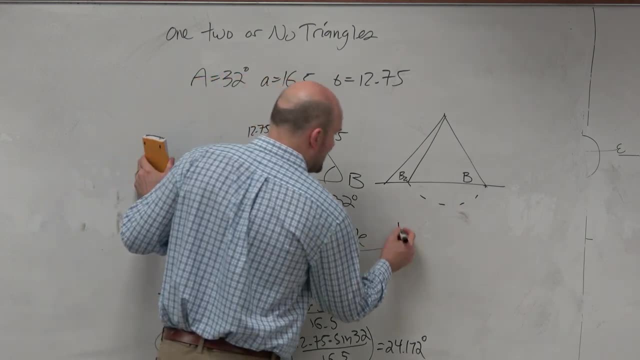 there would be another triangle, but it would have to be obtuse, Correct, Yes, So how? How do we figure out what b2 would be? So what you do is you take this as b to find b2 or to find this possible second triangle. 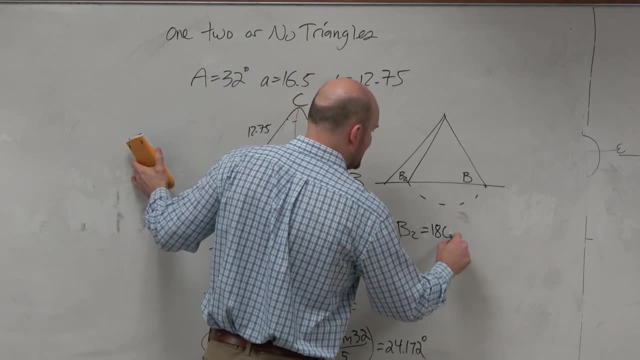 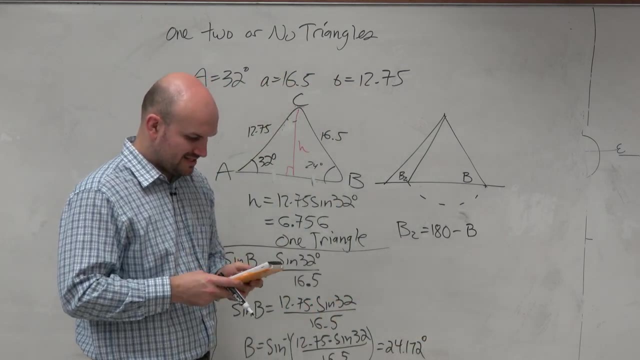 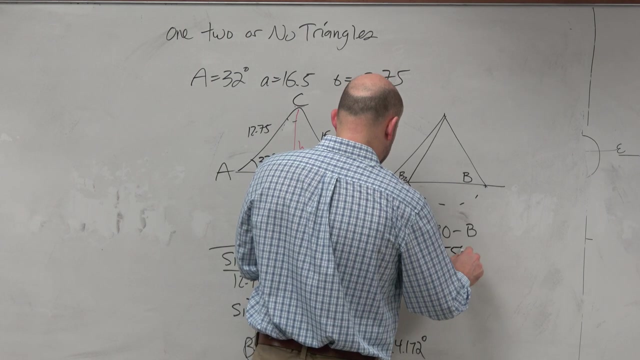 or angle in the second triangle. All you need to do is take 180 minus b, minus your b. So I just take 180 minus my last answer, or you could store it if you wanted to, And I get 155 degrees 0.83.. 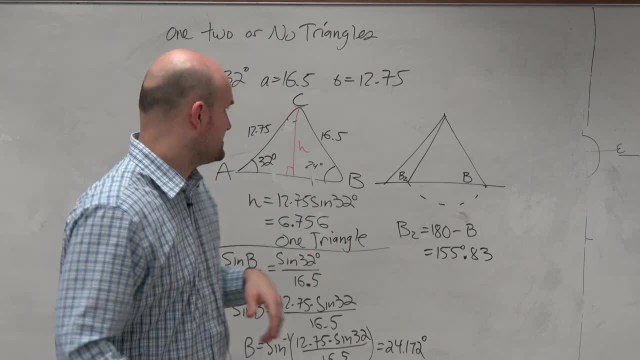 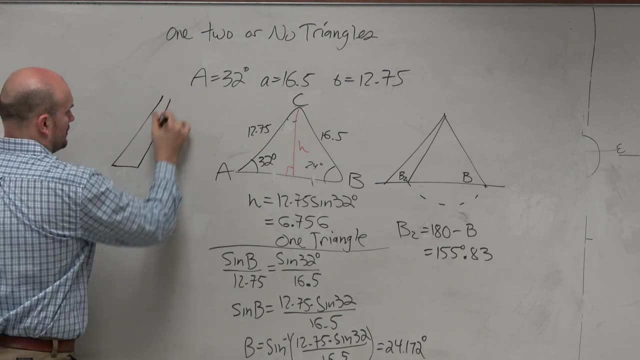 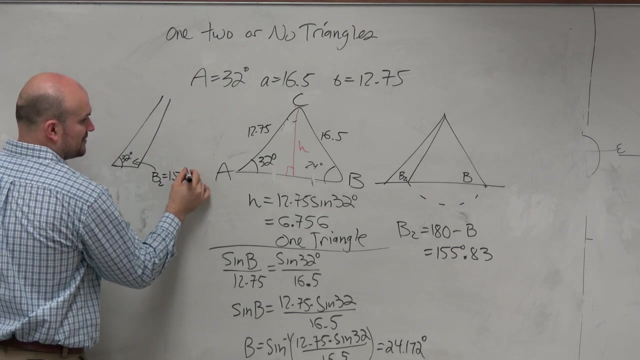 Now, here is the heart, Here's the thing I want you to understand. Does it make sense for me to have another triangle? Does it make sense for me to have another triangle where a is 32 degrees and b is b2 is 155 degrees roughly? 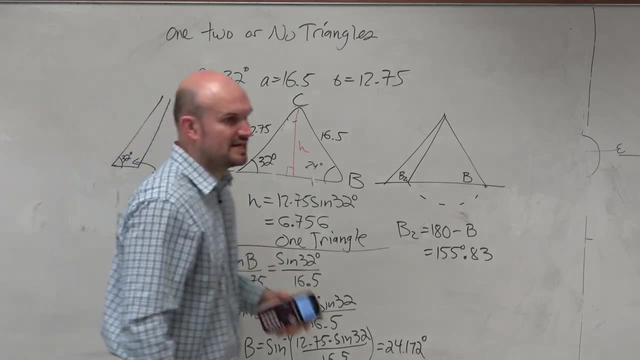 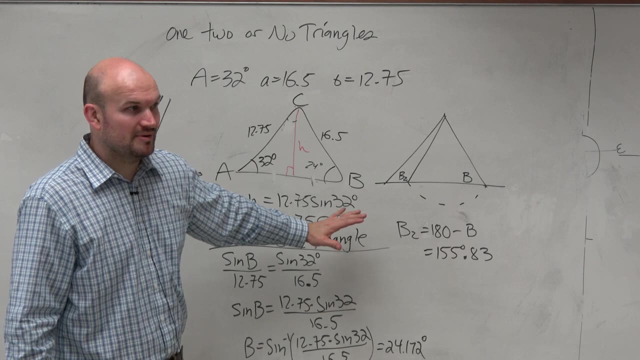 0.83.. Do those numbers make sense for a second triangle? No, because they're over 180, right, So you can do the h stuff, which I prefer, but I'm telling you you guys don't need to like. 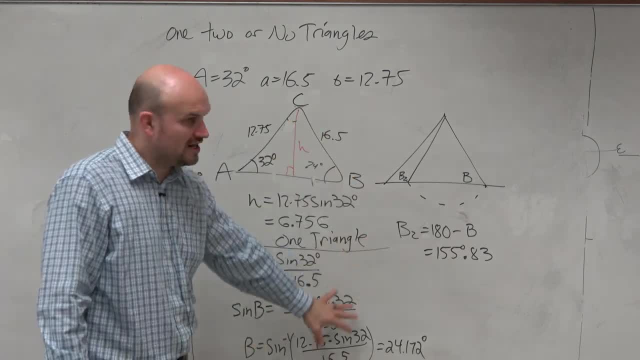 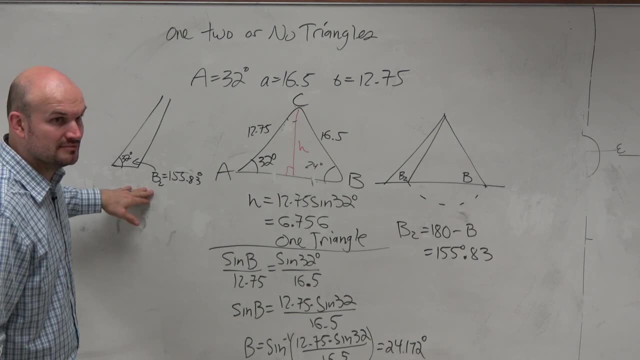 if you get stuck on it, just do the law of sines, figure out your missing angle, subtract it from 180.. If it doesn't work, then there's only one triangle right. If you do the law of sines and you get an error when you compute it, 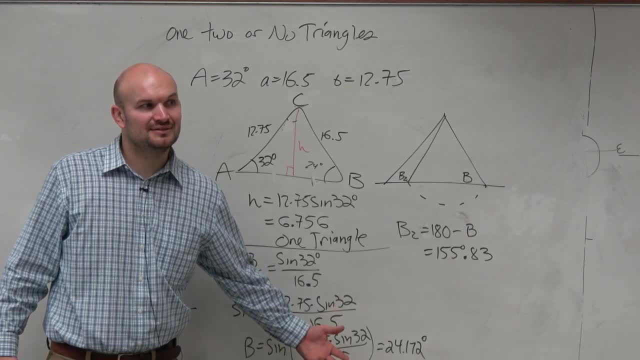 you either typed in something wrong or no triangle exists, okay. So how would then? So you might say: well, Mr McGlogin, how does the two?